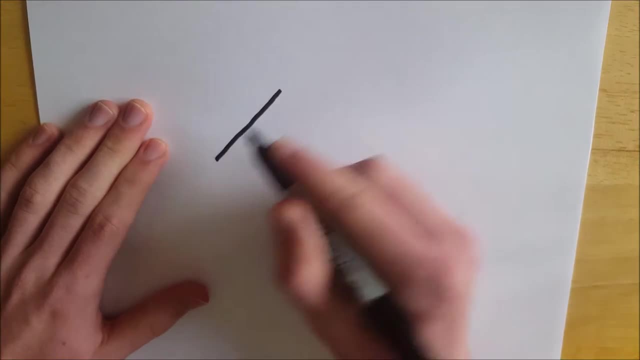 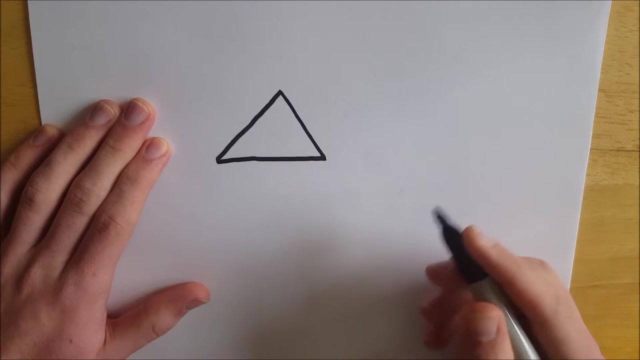 So let's construct. it's pretty easy, so it shouldn't take too long. Let's construct our isosceles triangle, something like that. I'm a very bad artist, so excuse me for all of my sketches on this channel. 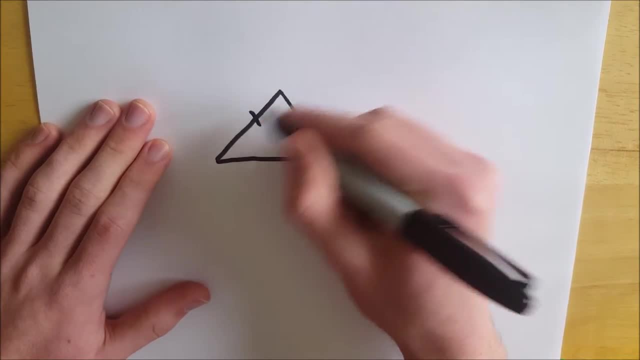 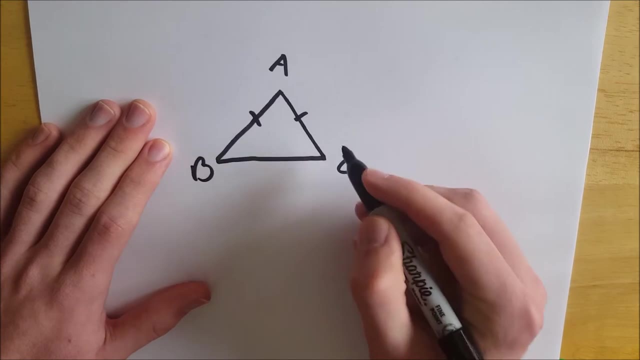 So it's an isosceles triangle, so we're going to have this side congruent to this side. I might as well label this A, B and C, So side AB is congruent to side AC, and then we're going to drop the altitude. 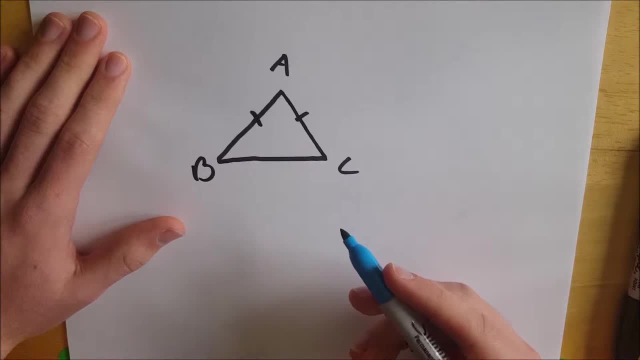 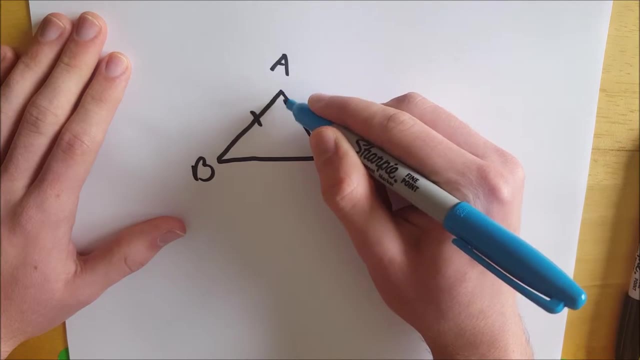 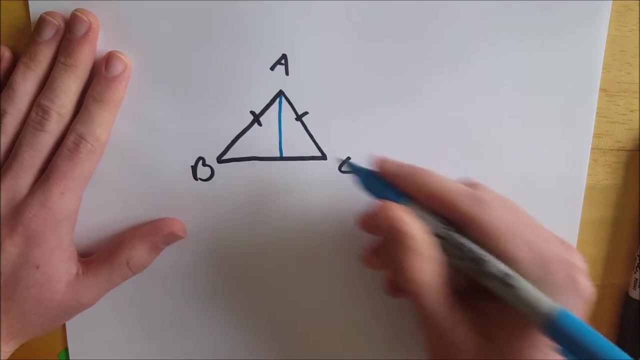 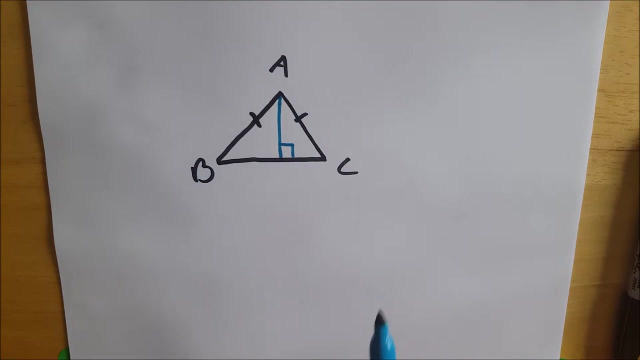 And, of course, when we're talking about the altitude of an isosceles triangle cutting two congruent triangles, we're talking about the altitude that has a vertex adjacent to the two congruent sides, so this one here. So the altitude goes from A down to side BC and is perpendicular to this side, And it's perpendicular over here as well. not going to bother writing that in because it looks gross. 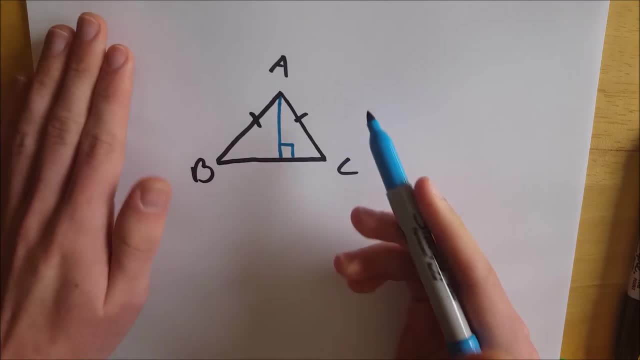 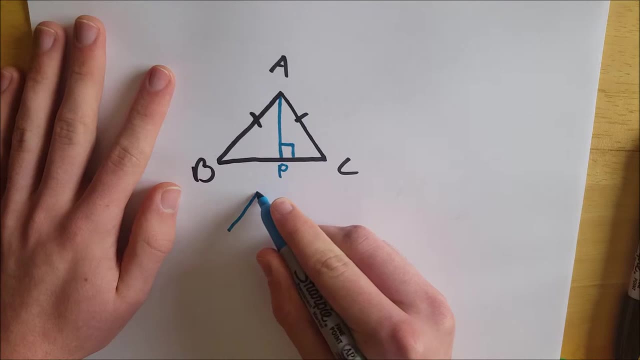 Of course they don't look congruent because I've done a poor job sketching it, but now we know that this triangle AB, we're going to call this point P. So now- and this is not to scale, of course, PAB, this right triangle that we've just cut, we're just shifting. 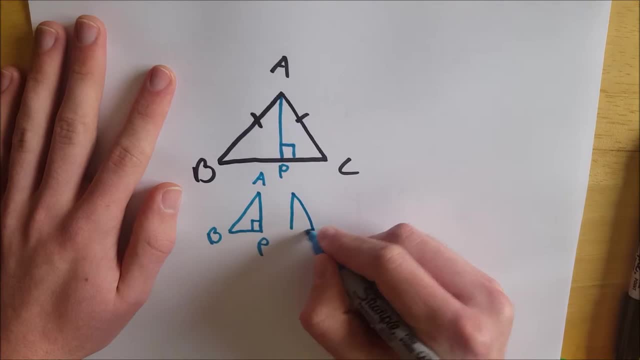 We're just shifting it over here- is congruent to triangle. so triangle ABP congruent to triangle ACP. And why is that? Well, we know that this side is congruent to this side because it's an isosceles triangle. that's how we drew it. 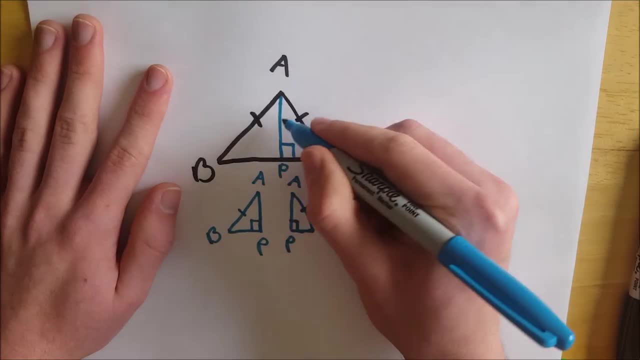 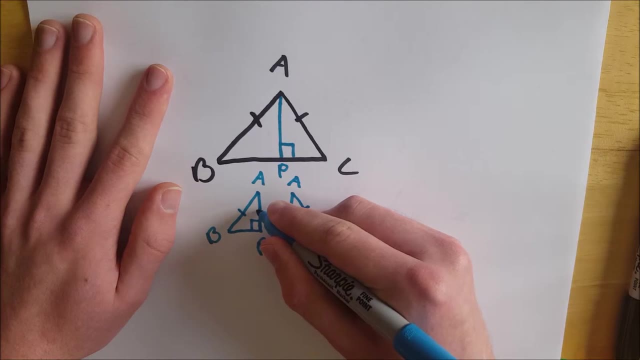 AB is congruent to AC and we know that this side, right here, AP is congruent to this side because this side is AP. So that's you know there. It's a reflexive property, it's congruent to itself. 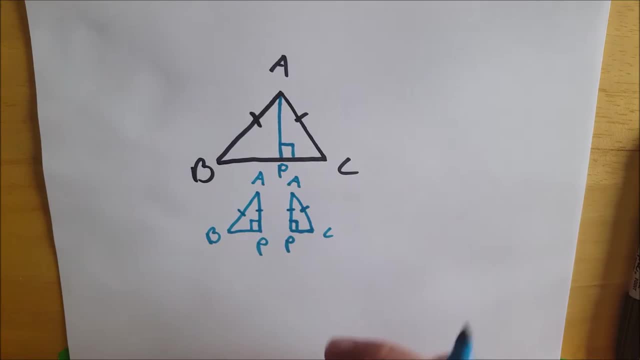 And so then, just like that, we've got the hypotenuse leg theorem for right triangles giving us congruency. So then we get that triangle. I'll write this out in black: triangle ABP by hypotenuse leg is congruent to triangle ACP. 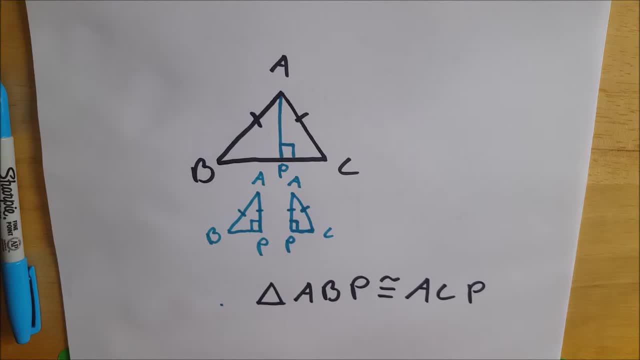 So it's pretty simple. So the altitude of an isosceles triangle That is adjacent to or that has a vertex adjacent to the two congruent sides cuts that isosceles triangle into two congruent right triangles, which we see here.